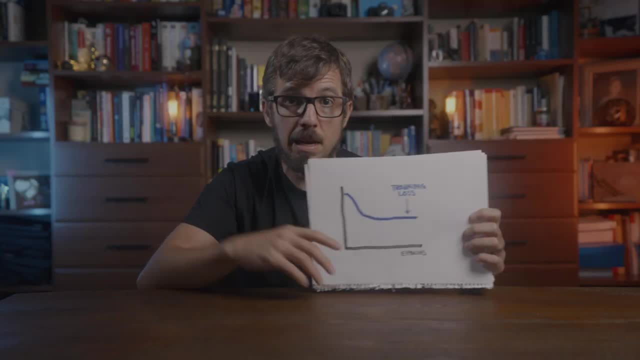 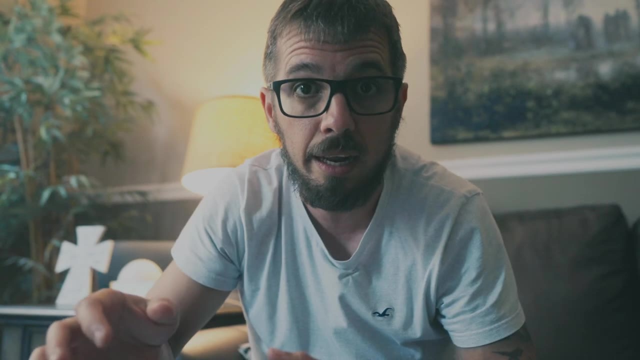 Lots of pictures. These are learning curves And, by the way, hey, me from the future here, including the haircut. if you're looking for something you can learn over a weekend, take a look into plotting and interpreting learning curves. That's a crucial skill you. 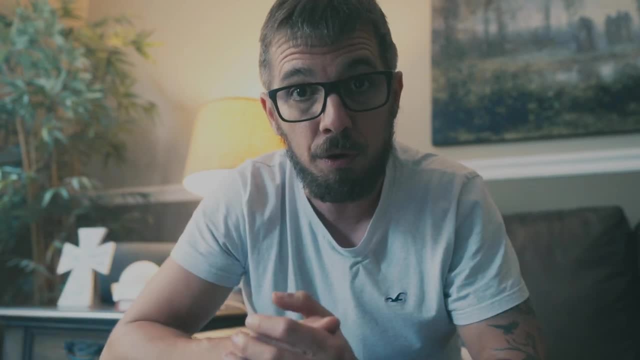 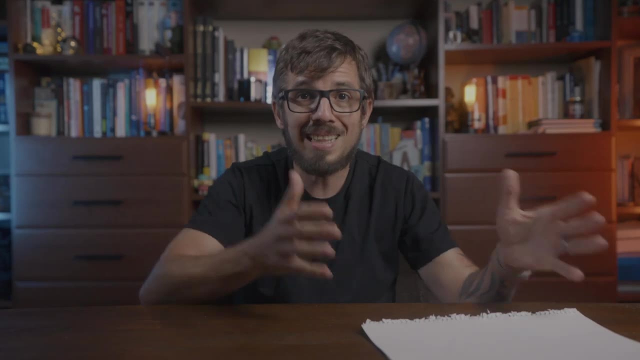 can build really, really quick. that will be fundamental for you. Let's get back to the video. Finally, I'll show you the learning curves of two models, each having a specific problem, something that happens every day. So, to get this started, think about a school, a teacher, 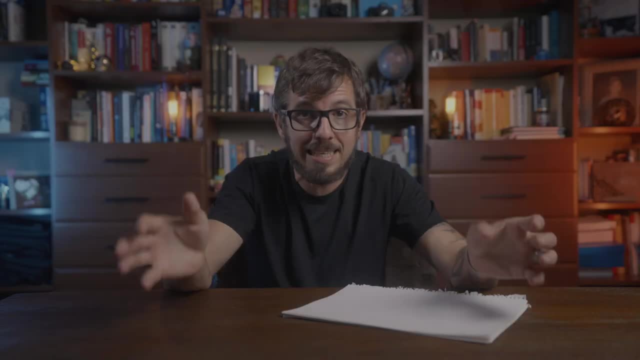 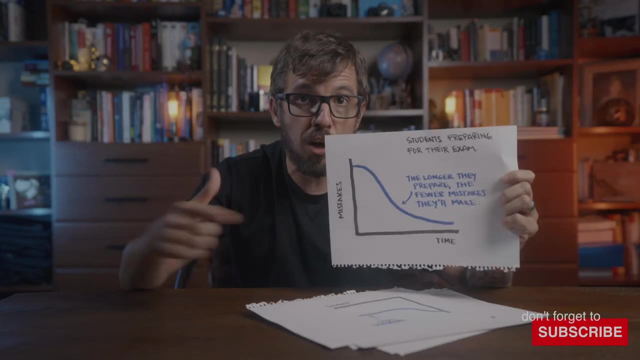 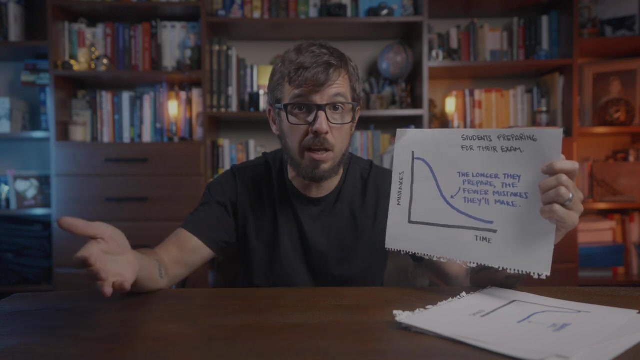 a set of questions you must study for every exam. At the end of the year the teacher publishes this, This chart. it shows the number of mistakes students made in relation to how long they had to study. The longer the students prepare, the better they do. That makes sense. Every teacher. 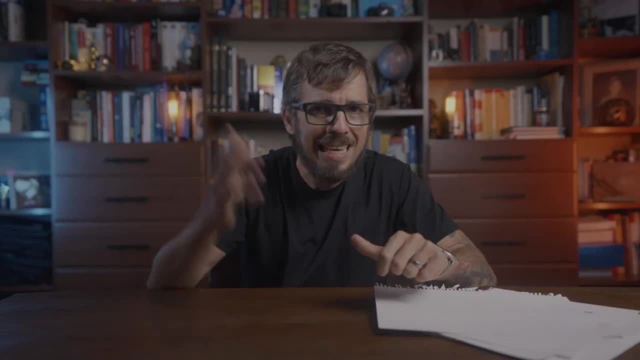 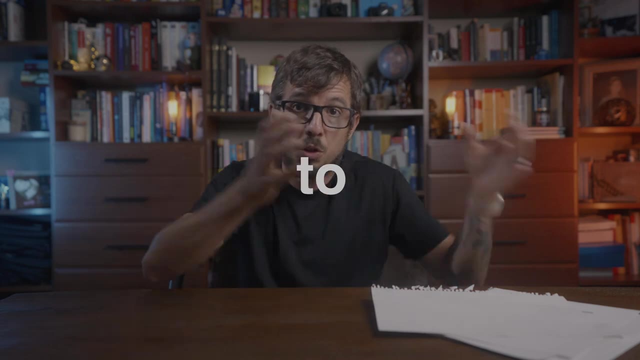 out there wants their students to learn the material. They don't want students to optimize for the exam. They want to build knowledge that will later generalize to situations they'll see outside the classroom. We can connect this idea with the way we train models in machine learning. 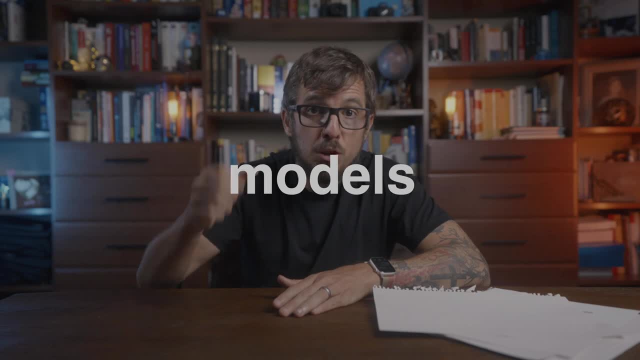 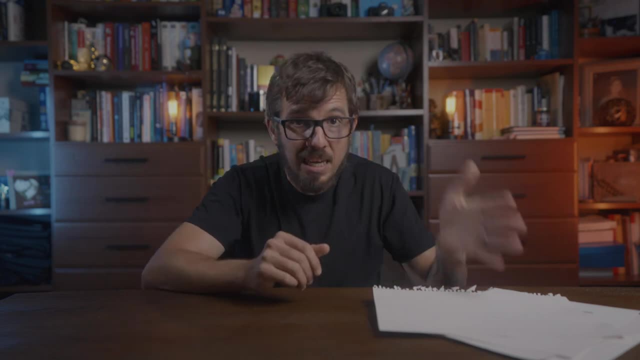 The same principles apply. We want machine learning models to learn and generalize what they know to solve samples outside the training dataset. A model that doesn't learn or can't generalize to new data is a useless model. We use two terms to refer to these models. 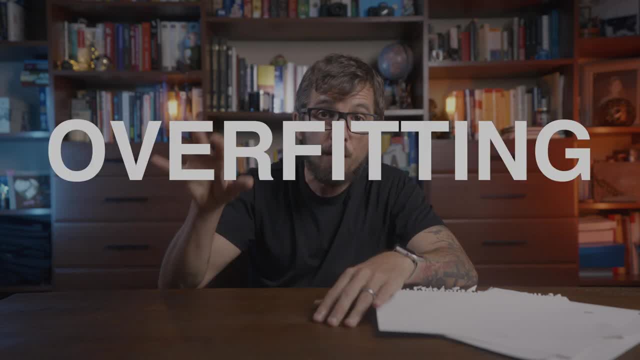 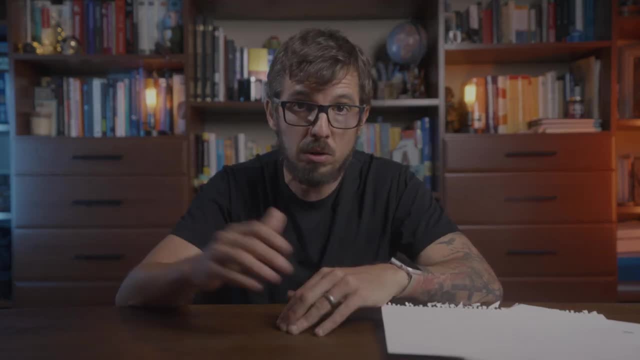 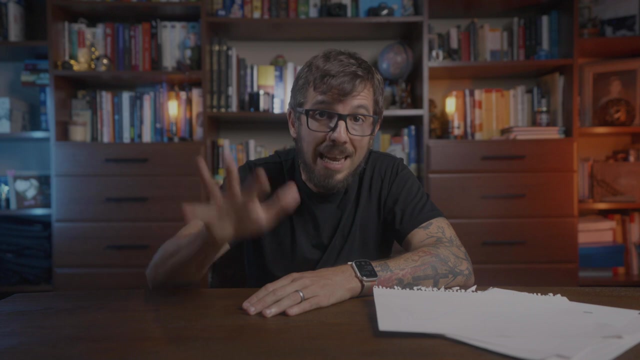 underfitting if a model didn't learn, and overfitting if a model doesn't generalize to unseen samples. Both cases lead to useless models. Fortunately, there are many different ways to deal with underfitting and overfitting, But before we can do anything, we need to identify. 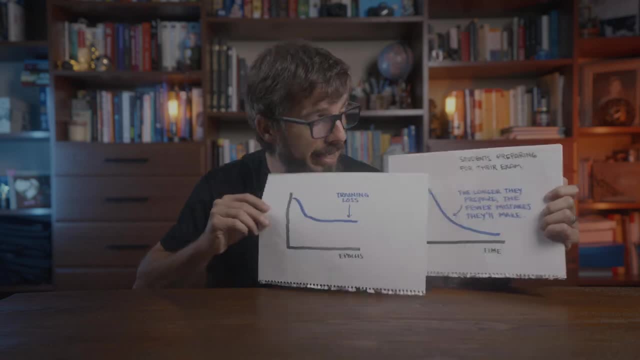 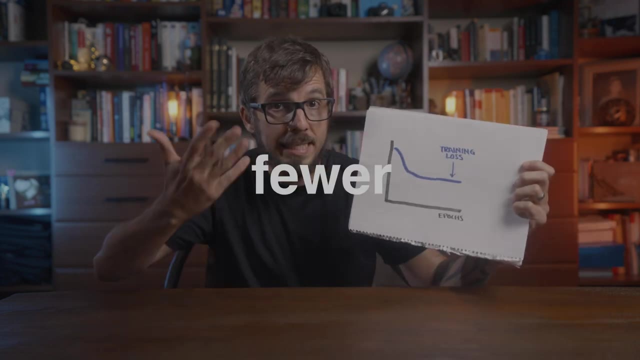 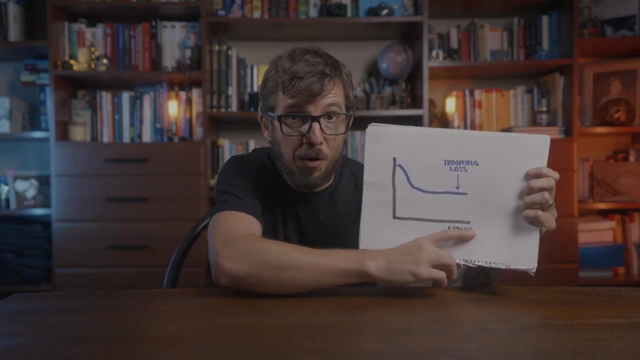 them. So let's look at this chart, Very similar to the first one. Instead of mistakes, we have the model's loss- Similar concept: The fewer mistakes the model makes, the lower the loss is going to be, And that's what we want. Instead of time, here we talk about epochs. 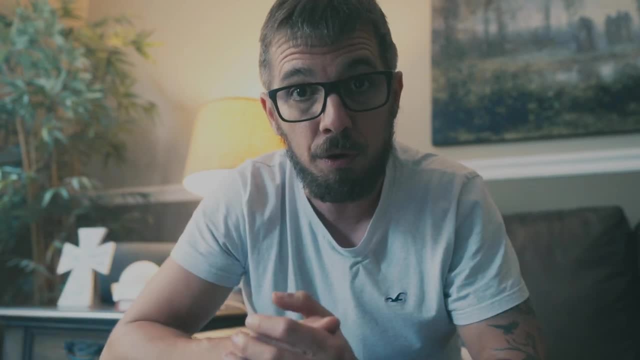 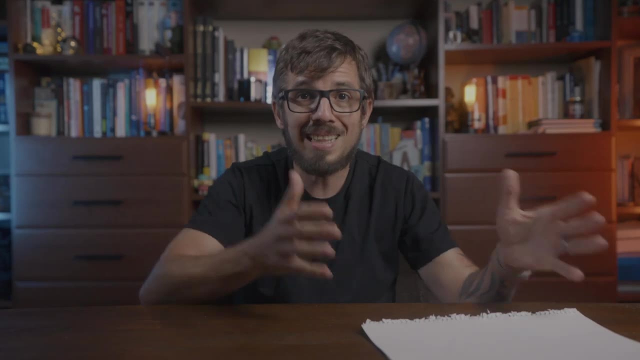 can build really, really quick. that will be fundamental for you. Let's get back to the video. Finally, I'll show you the learning curves of two models, each having a specific problem, something that happens every day. So, to get this started, think about a school, a teacher, 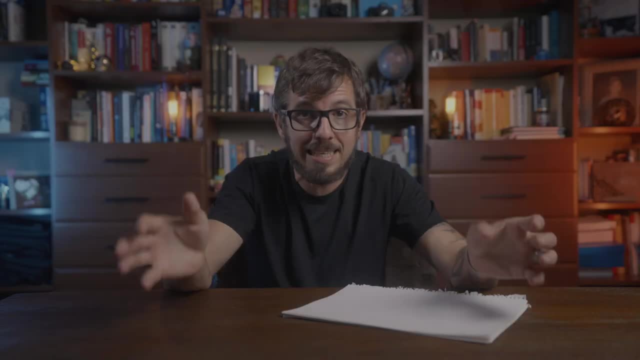 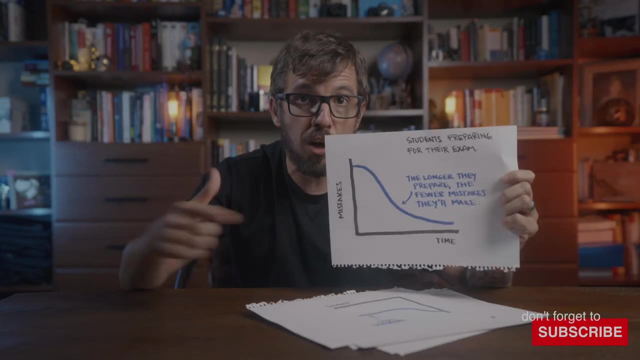 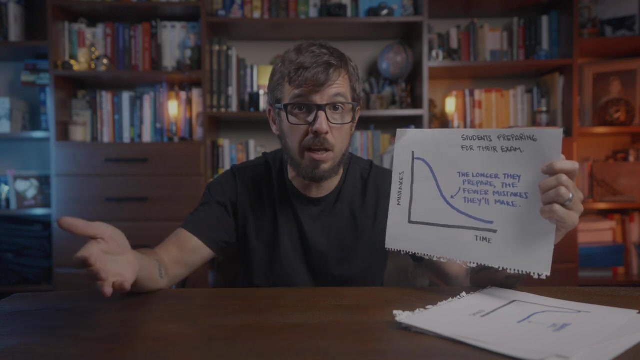 a set of questions you must study for every exam. At the end of the year the teacher publishes this, This chart. it shows the number of mistakes students made in relation to how long they had to study. The longer the students prepare, the better they do. That makes sense. Every teacher. 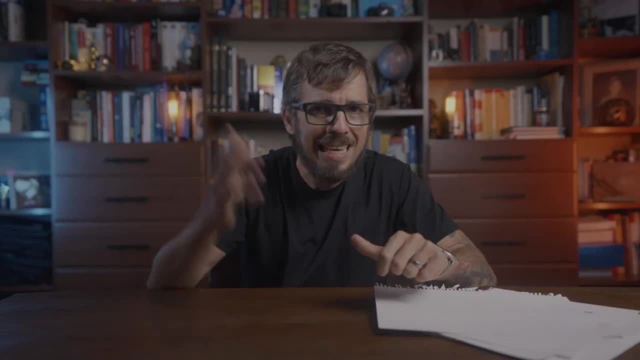 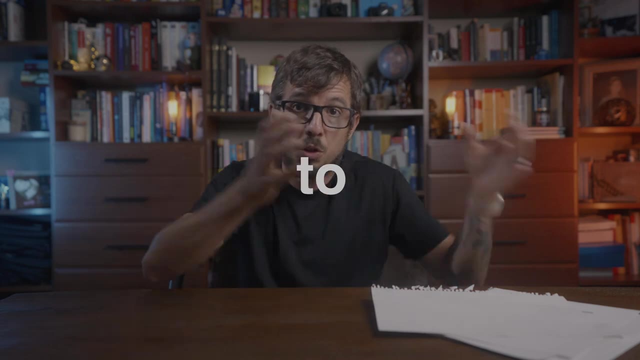 out there wants their students to learn the material. They don't want students to optimize for the exam. They want to build knowledge that will later generalize to situations they'll see outside the classroom. We can connect this idea with the way we train models in machine learning. 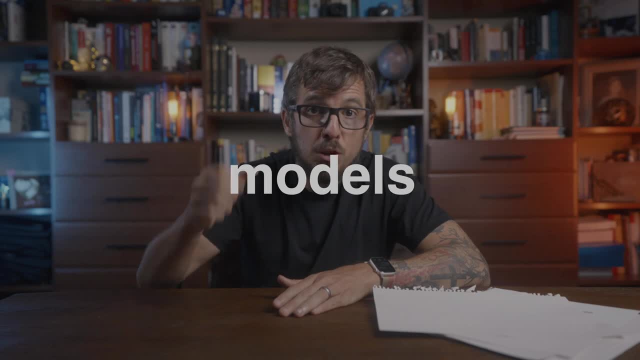 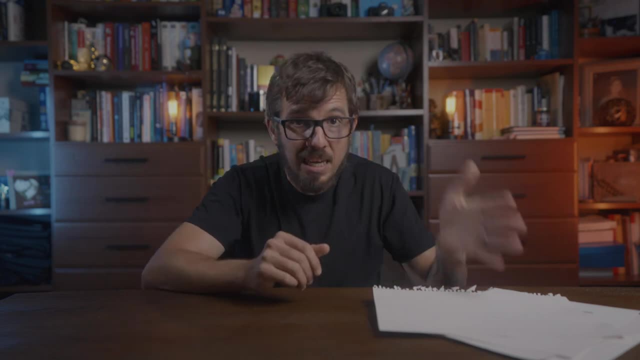 The same principles apply. We want machine learning models to learn and generalize what they know to solve samples outside the training dataset. A model that doesn't learn or can't generalize to new data is a useless model. We use two terms to refer to these models. 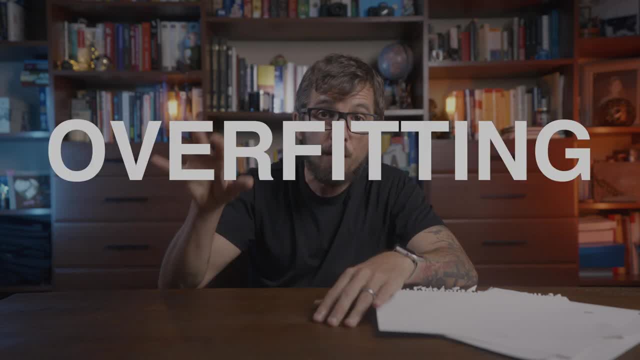 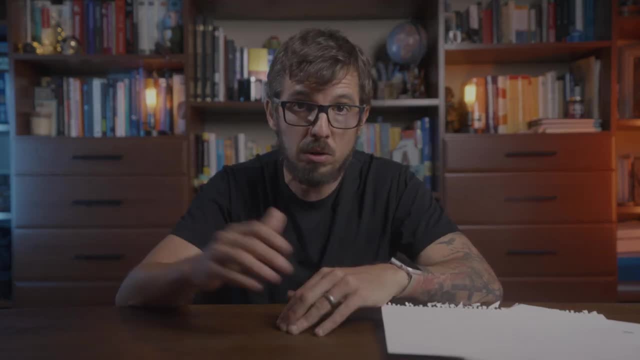 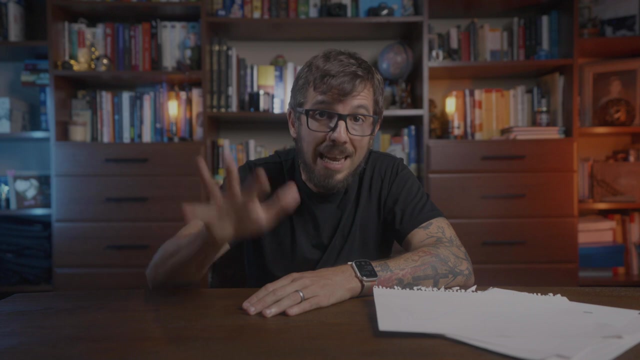 underfitting if a model didn't learn, and overfitting if a model doesn't generalize to unseen samples. Both cases lead to useless models. Fortunately, there are many different ways to deal with underfitting and overfitting, But before we can do anything, we need to identify. 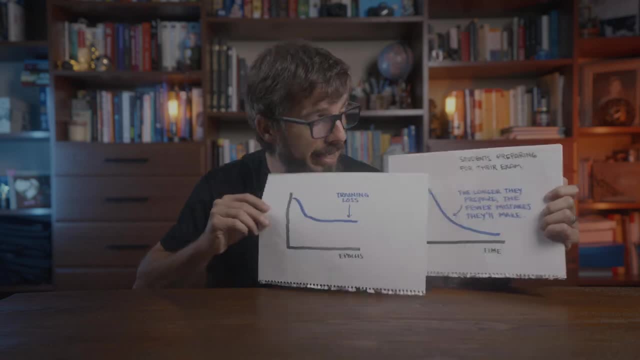 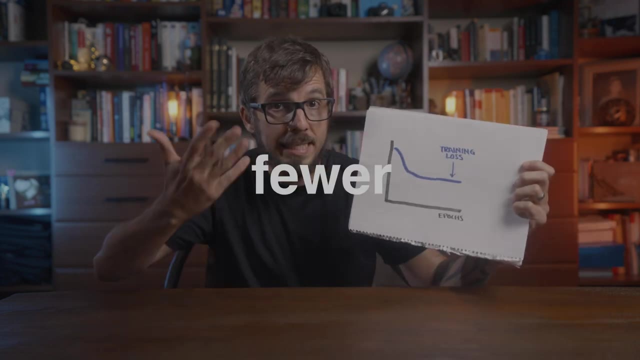 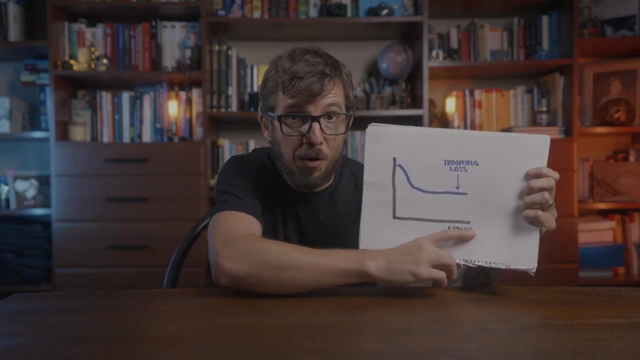 them. So let's look at this chart, Very similar to the first one. Instead of mistakes, we have the model's loss- Similar concept: The fewer mistakes the model makes, the lower the loss is going to be, And that's what we want. Instead of time, here we talk about epochs. 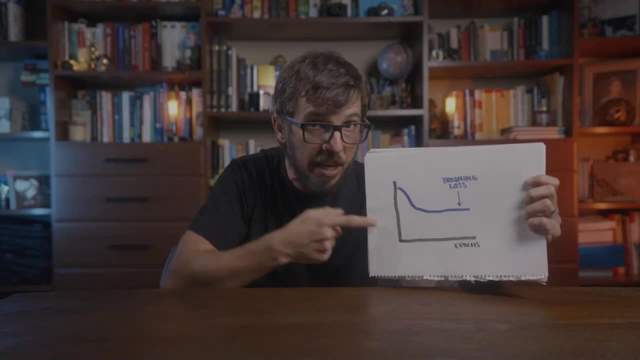 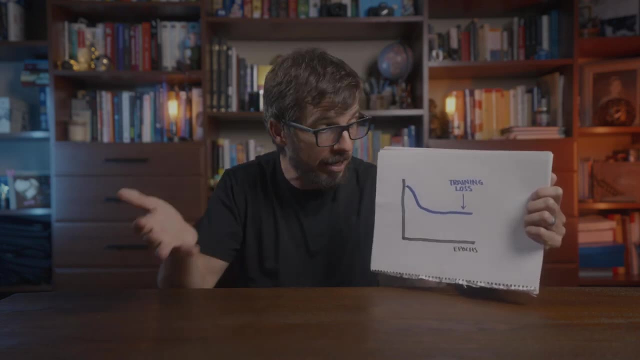 which are the number of iterations we spend training this model. We call this a learning curve. They are crucial for diagnosing underfitting and overfitting in machine learning models. I want you to notice something important in this chart. This is the. 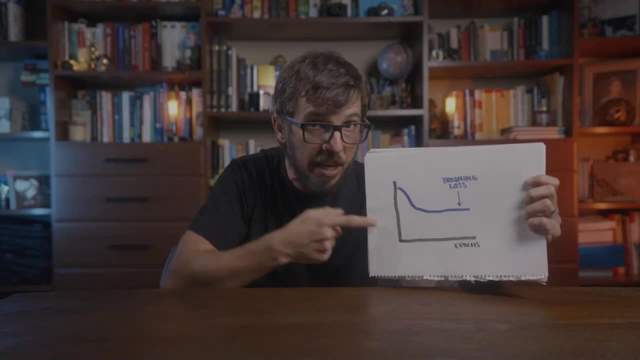 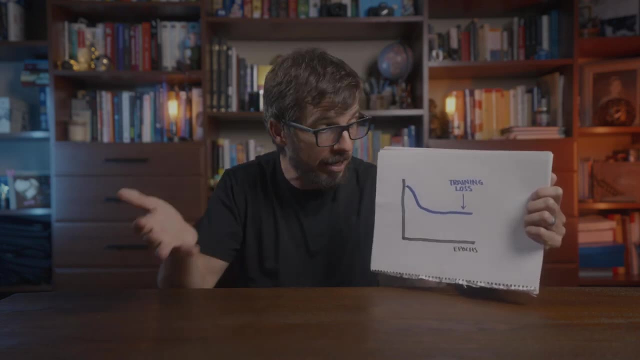 which are the number of iterations we spend training this model. We call this a learning curve. They are crucial for diagnosing underfitting and overfitting in machine learning models. I want you to notice something important in this chart. This is the. 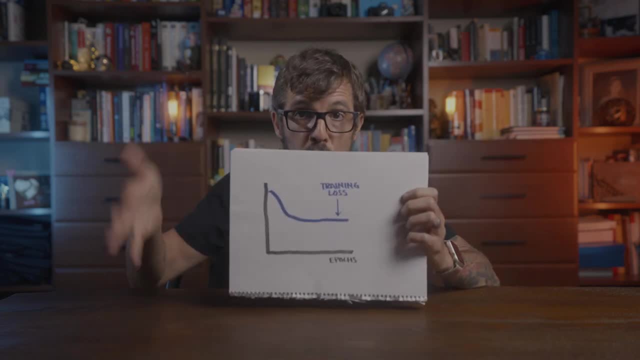 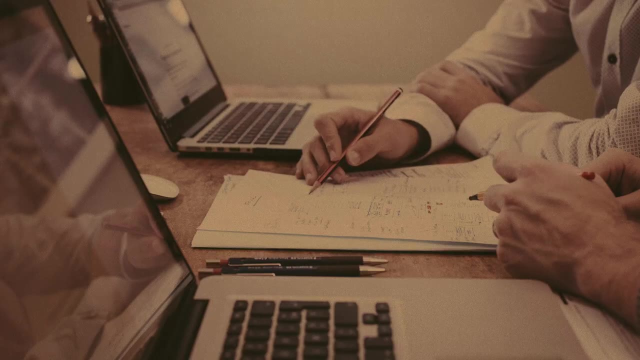 training: loss of the model. We are measuring the model's learning ability on the same data we use to train it. Going back to the student's analogy, imagine the teacher using the same questions they discussed in class to evaluate students during the exam. Presumably. 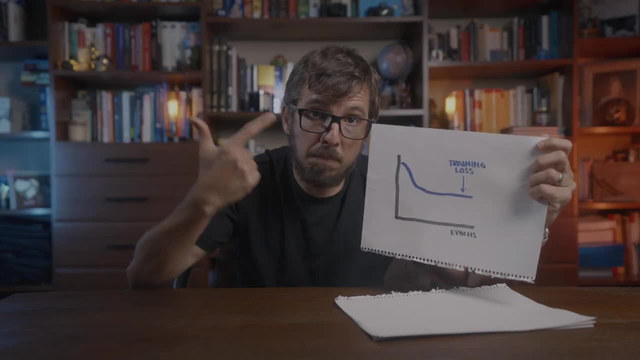 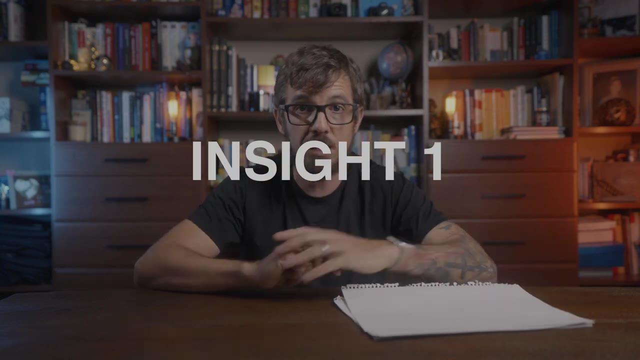 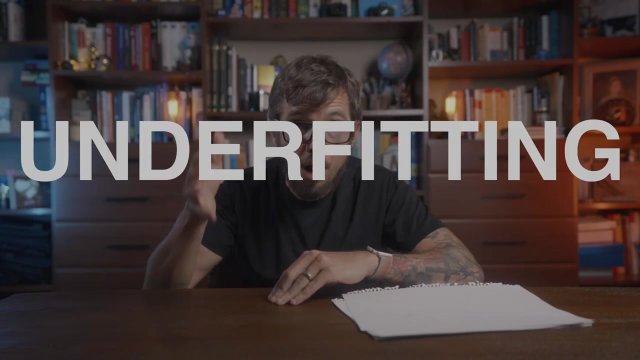 students could memorize the answers and do great. This model has every possible advantage to do well, and yet the loss is not good. You know why? Here is the first insight of this video: A high training loss indicates the model doesn't fit the data correctly. We call this underfitting. Here is 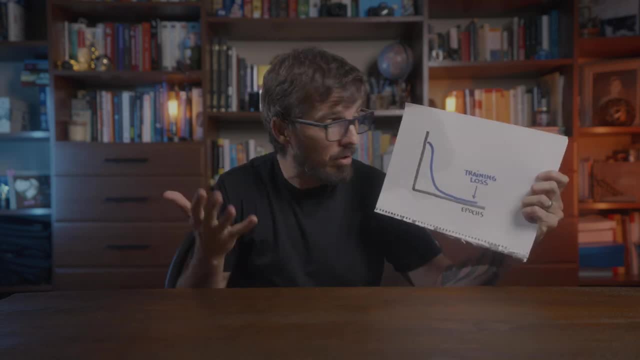 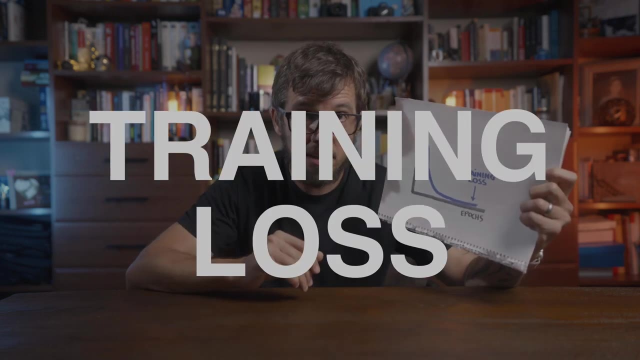 a different story. The training loss here is low. so we know this model is not underfitting, But can we say this is a good model? Remember, this is the training loss. This is similar to the teacher testing students on the same questions they saw during class. If those 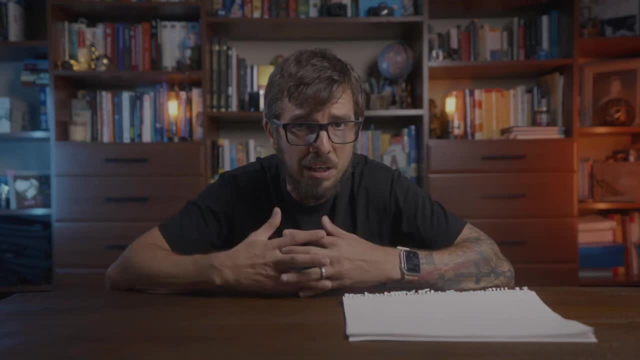 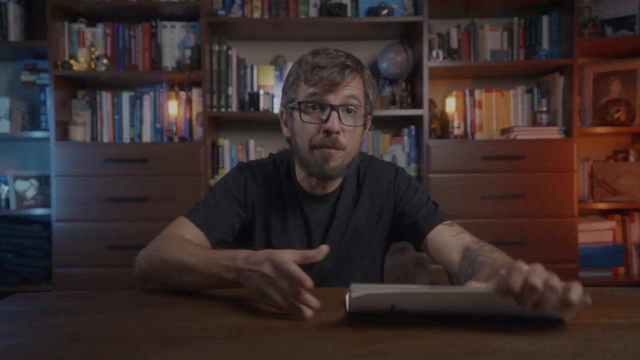 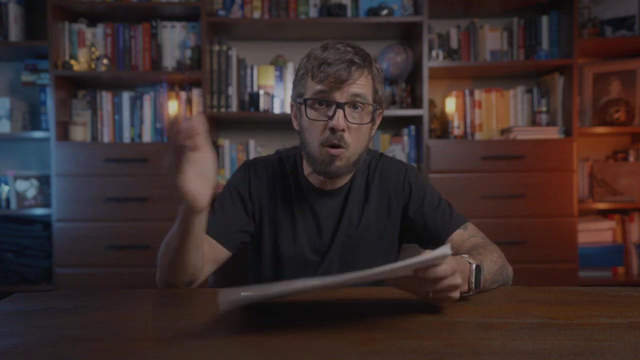 students aced the exam. can we say they learned the material? No, we cannot. Maybe they just memorized every answer and didn't learn anything. We need more information to decide whether this is a good model. Every teacher will create an exam with different questions from the ones. 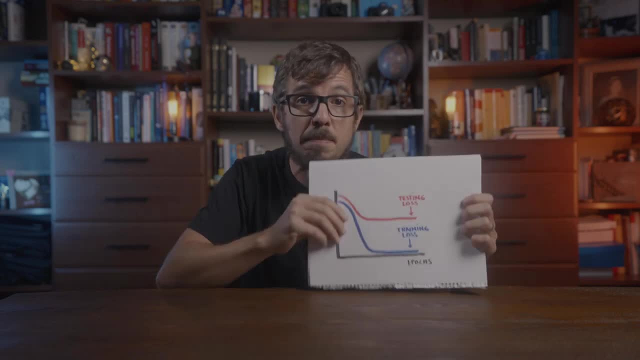 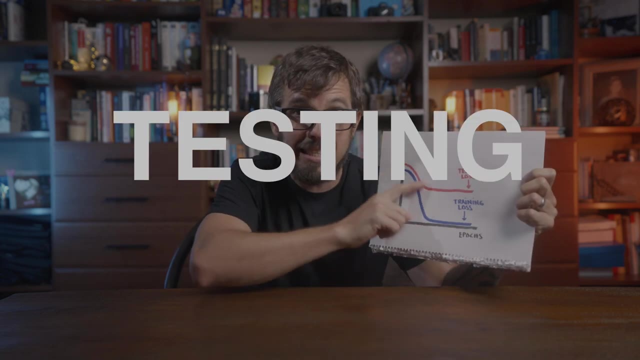 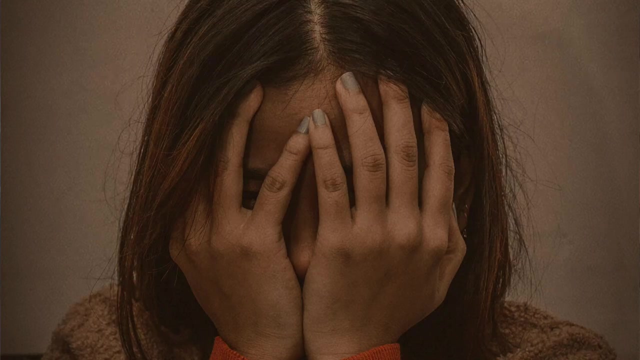 students saw. We can use the same idea and evaluate the model on a different data set. We now have two learning curves: One training loss and one testing loss. The testing loss here is high. Students did well on the questions they knew beforehand but did horrible. 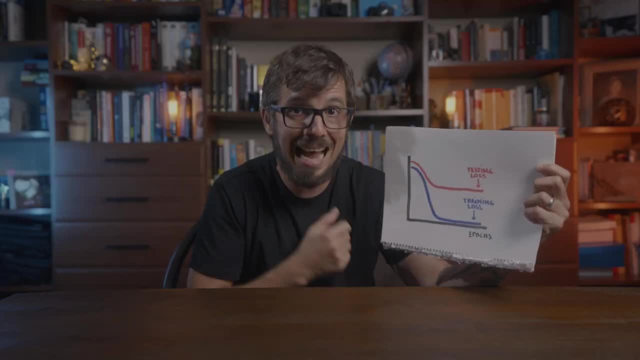 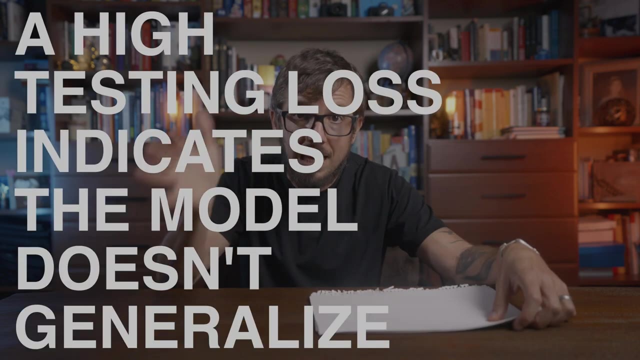 on the new questions. So this is not a good model. And here is the second insight: A high testing loss indicates the model doesn't generalize well. Whenever this happens, we say the model is overfitting. Okay, not this. Here are good-looking. 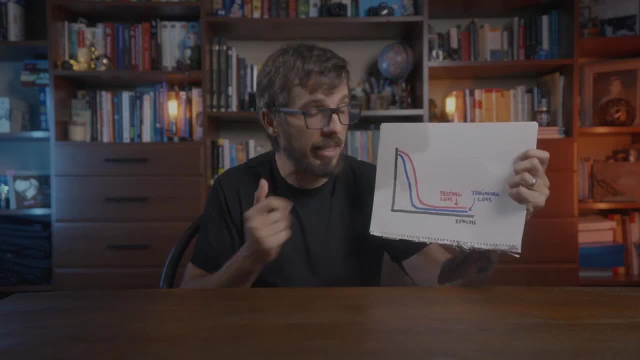 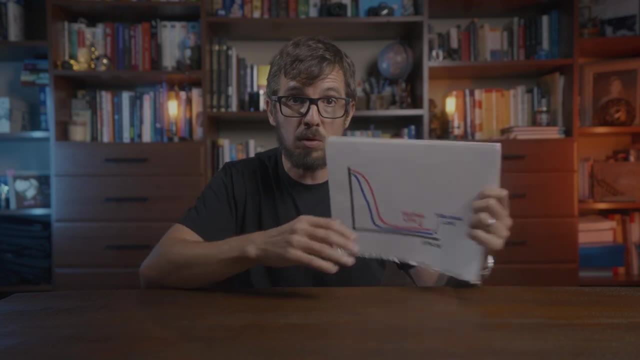 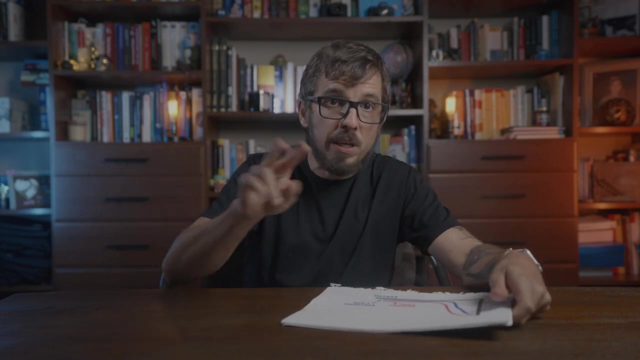 curves. Low training loss: it means our model learns the training data well. Low testing loss: it means our model generalizes to unseen data. This is a well-fit model. No underfitting, no overfitting. This is what we want to see. Remember, I told you about two separate. 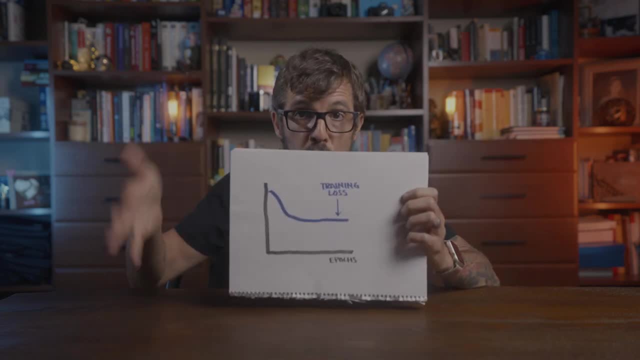 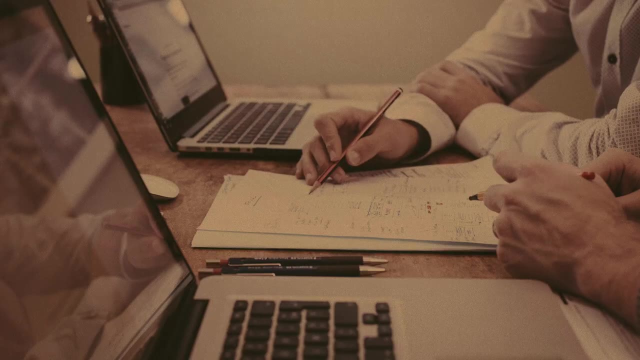 training: loss of the model. We are measuring the model's learning ability on the same data we use to train it. Going back to the student's analogy, imagine the teacher using the same questions they discussed in class to evaluate students during the exam. Presumably. 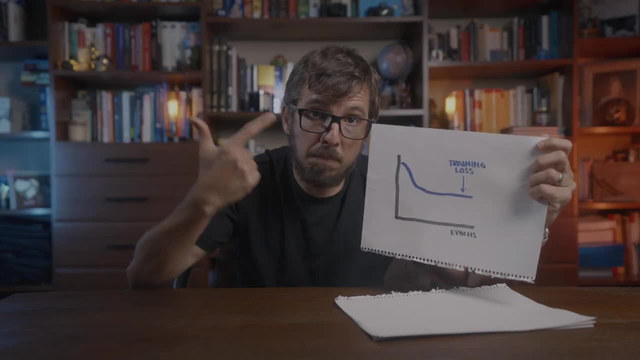 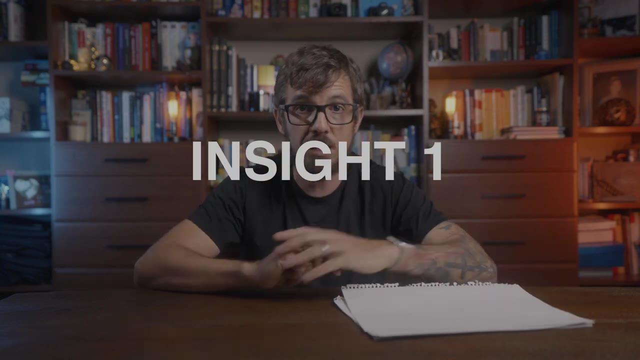 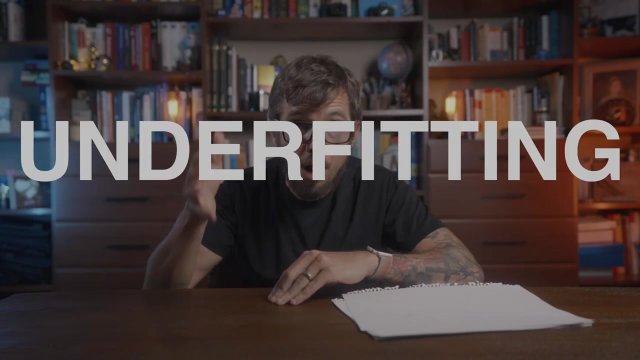 students could memorize the answers and do great. This model has every possible advantage to do well, and yet the loss is not good. You know why? Here is the first insight of this video: A high training loss indicates the model doesn't fit the data correctly. We call this underfitting. Here is 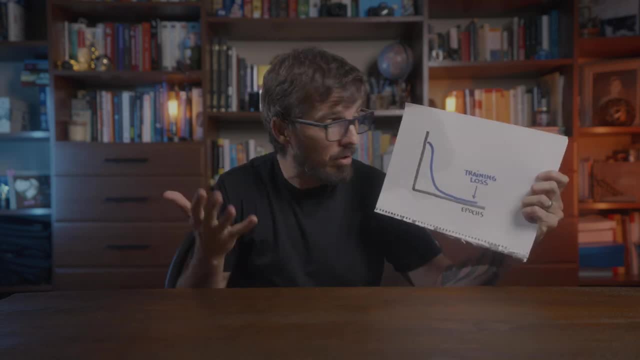 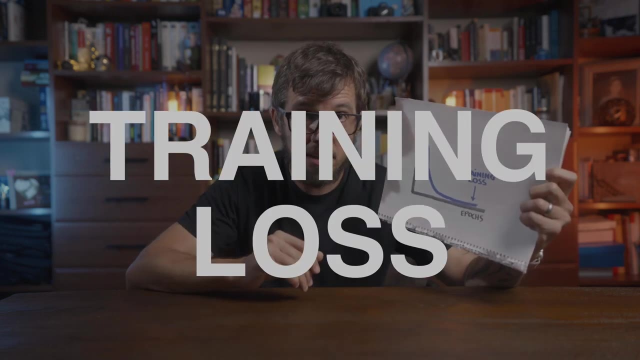 a different story. The training loss here is low. so we know this model is not underfitting, But can we say this is a good model? Remember, this is the training loss. This is similar to the teacher testing students on the same questions they saw during class. If those 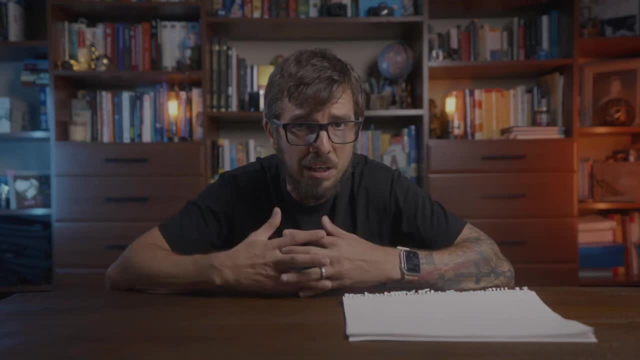 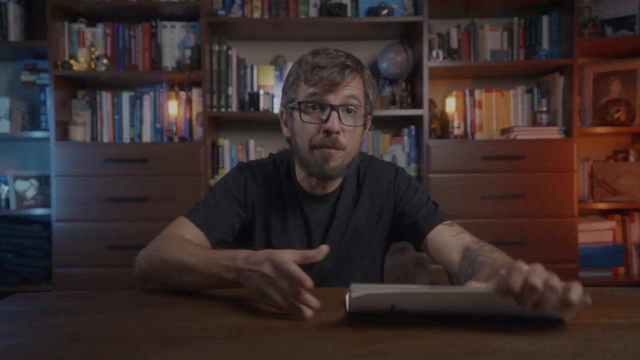 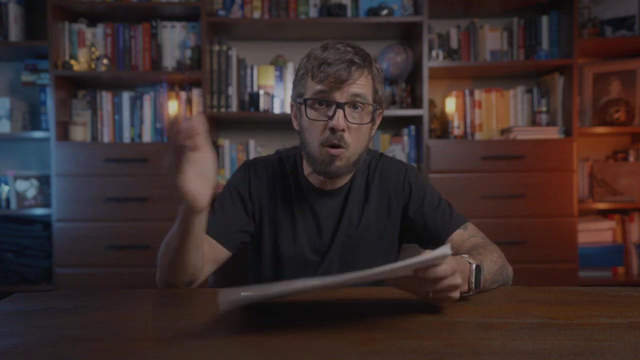 students aced the exam. can we say they learned the material? No, we cannot. Maybe they just memorized every answer and didn't learn anything. We need more information to decide whether this is a good model. Every teacher will create an exam with different questions from the ones. 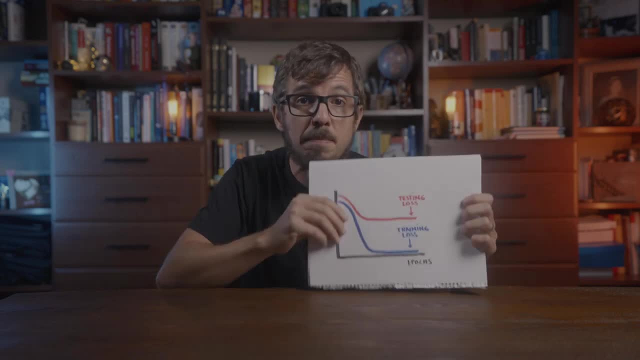 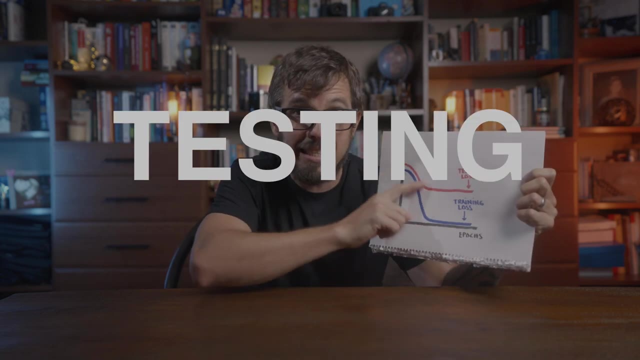 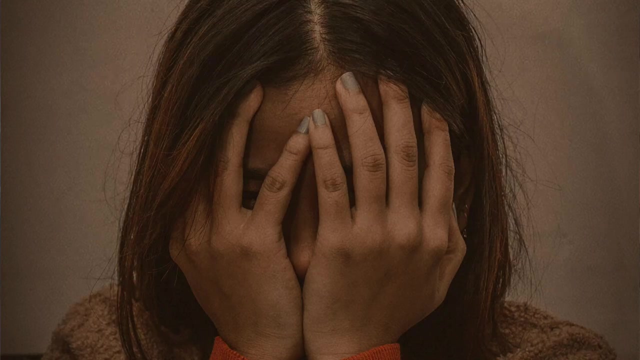 students saw. We can use the same idea and evaluate the model on a different data set. We now have two learning curves: One training loss and one testing loss. The testing loss here is high. Students did well on the questions they knew beforehand but did horrible. 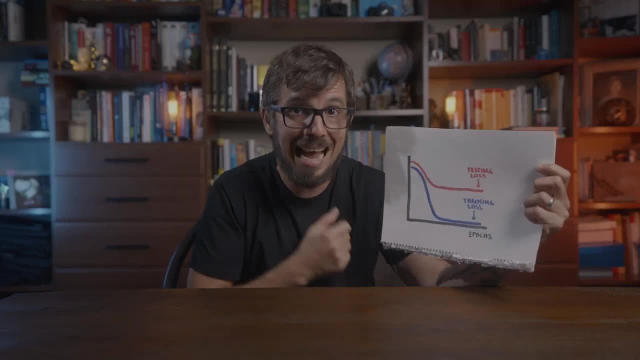 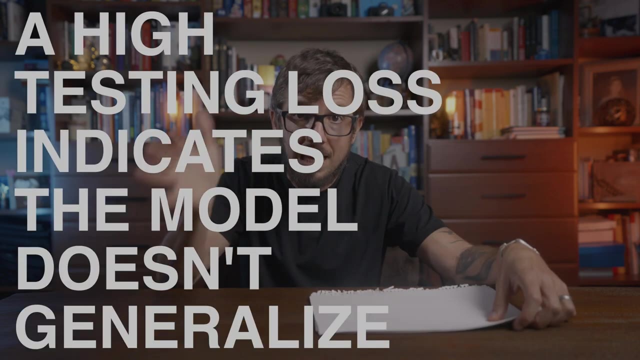 on the new questions. So this is not a good model. And here is the second insight: A high testing loss indicates the model doesn't generalize well. Whenever this happens, we say the model is overfitting. Okay, not this. Here are good-looking. 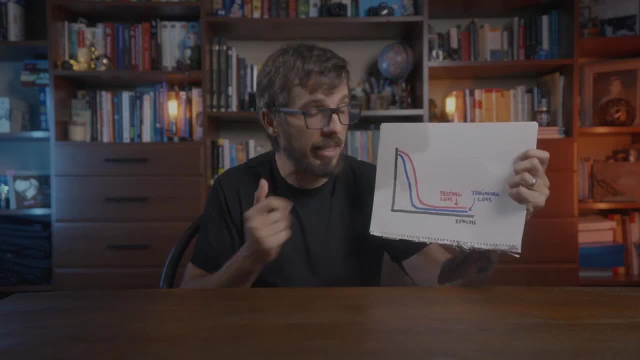 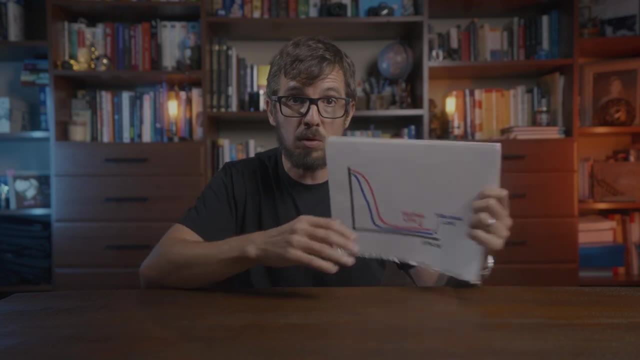 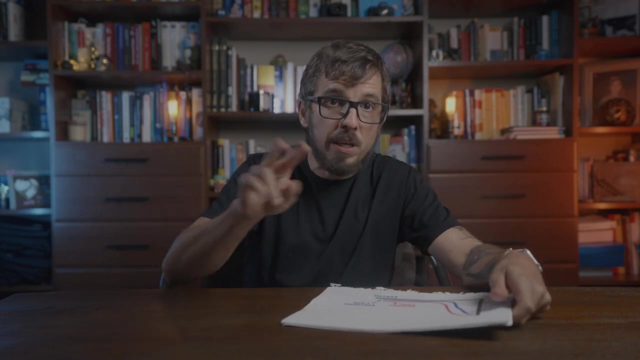 curves. Low training loss: it means our model learns the training data well. Low testing loss: it means our model generalizes to unseen data. This is a well-fit model. No underfitting, no overfitting. This is what we want to see. Remember, I told you about two separate. 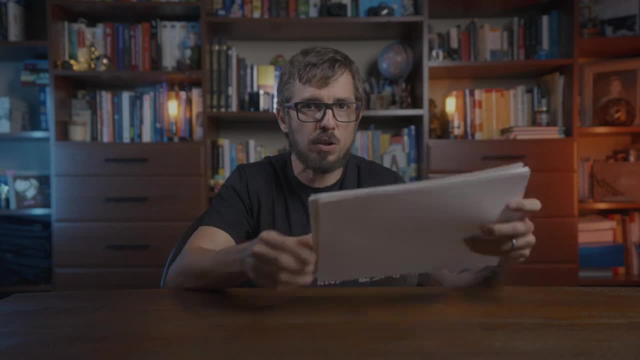 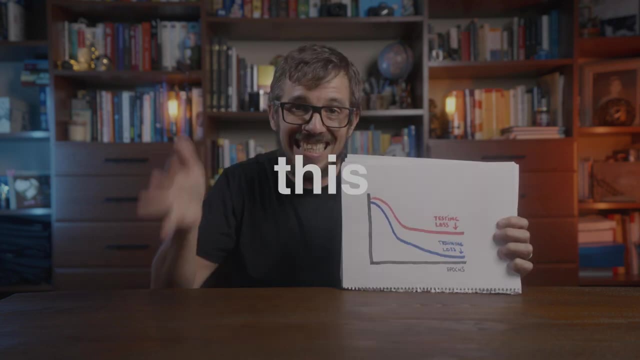 specific situations I wanted to show you. Here is the first one. These curves are decreasing. It looks like things are fine, but notice the gap between them. This happens whenever the model is low on the testing set, For example, there might be some differences between the.